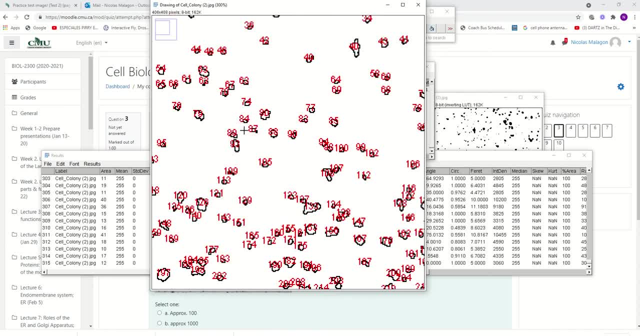 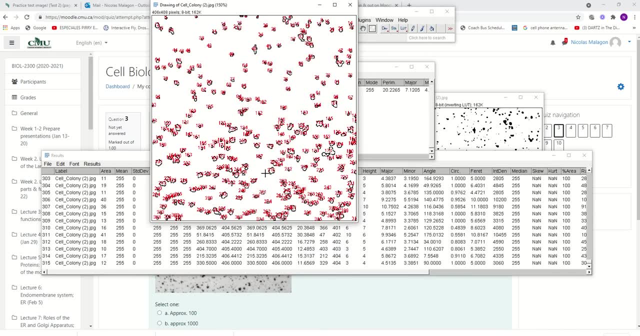 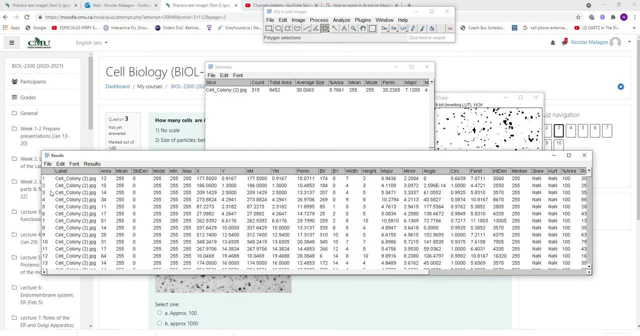 So here you can see all of them labeled. Here you see 74,, 84. There are so many and in this time this is not as useful, And here they give you the count. You can also in the other one, in this other results section they tell you how many there are And if you see the 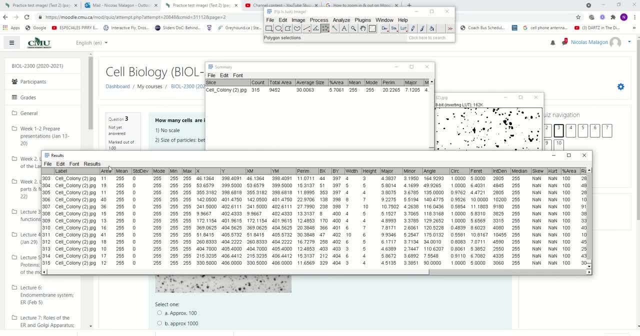 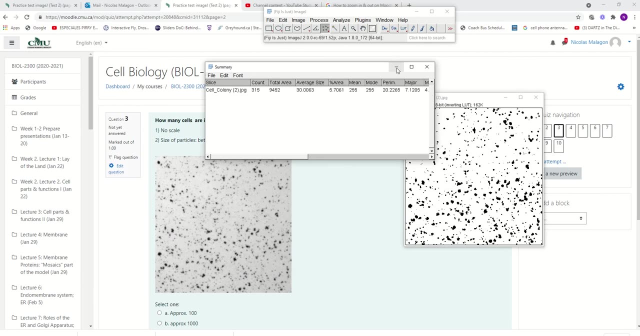 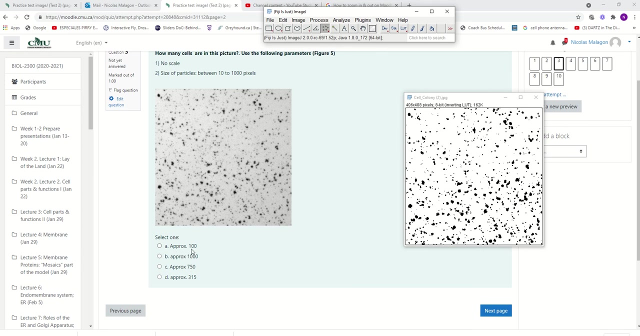 three hundred fifteen Here the area and pedometer High, with all the thing that you said that I might ask. So now we know that there is 350 in this size, So we they will say that there is approximately 100, 1000, 750 or 315.. So here the answer. 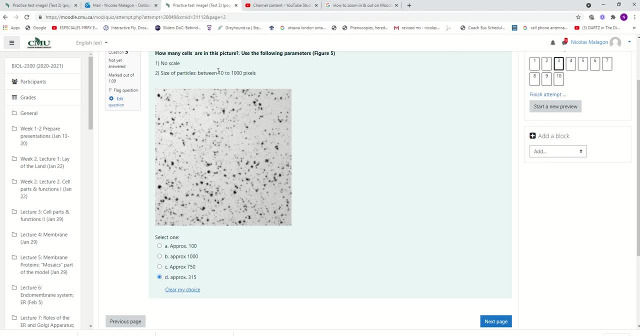 I don't see it. Okay, Well, we make it buy. So here it is. So here it's 50.. Well, here be 315. remember these parameters are very important. if I change, there is a different scale or there are different numbers of a different size, there will. 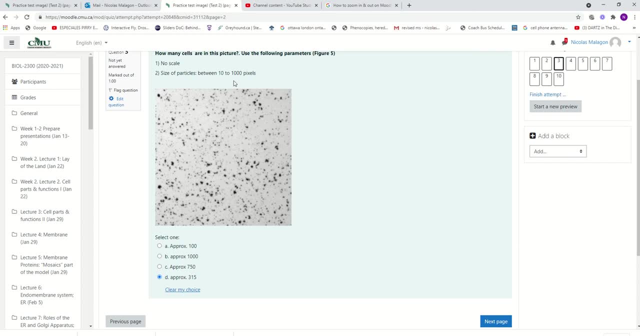 be different number. okay, if you have any question, send me an email and I will try to help you. 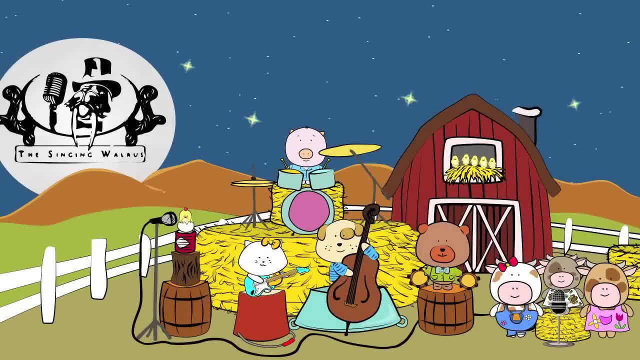 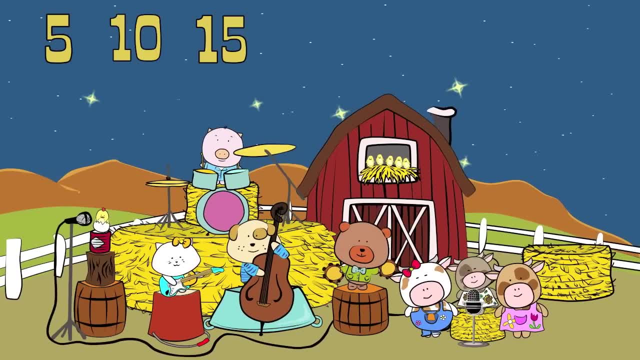 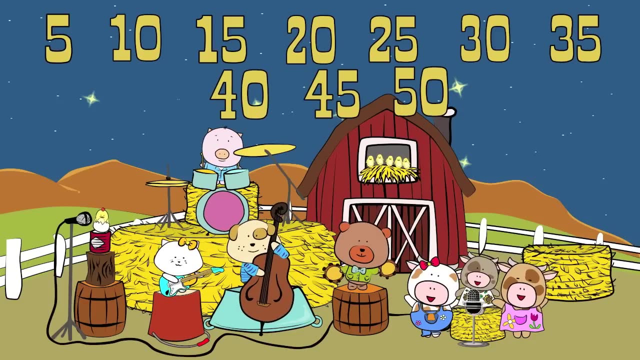 The Singing Walrus Counting by Fives: 5,, 10,, 15,, 20,, 25,, 30,, 35,, 40,, 45, 50. 5,, 10,, 15,, 20,, 25,, 30,, 35,, 40,, 45,, 50. 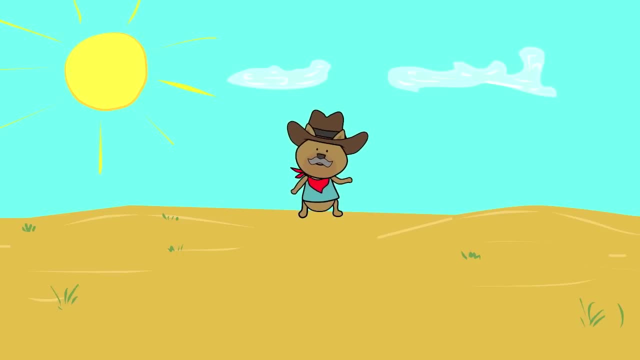 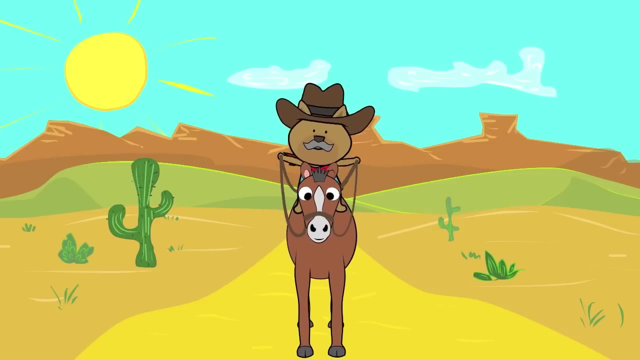 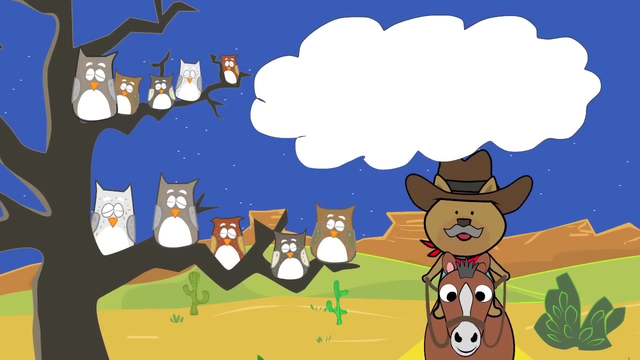 Billy is a cowboy, a cowboy with a horse. Billy goes to many places on his horse. of course, Billy travels all the time, even late at night. He likes to look around and count, and he likes to count by fives.